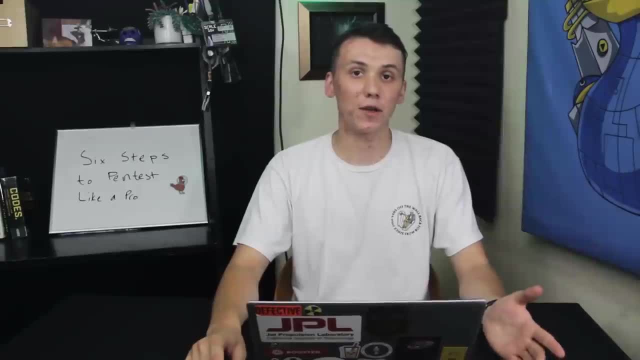 to be vulnerable. Stage four, exploitation, is arguably the most exciting phase of a penetration test. This is where we use all the intelligence that we've gathered in the previous three steps and apply it to exploit our targeted device. Now, this can vary widely based on the type of 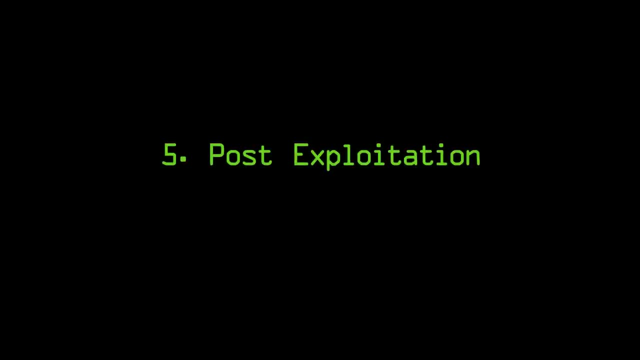 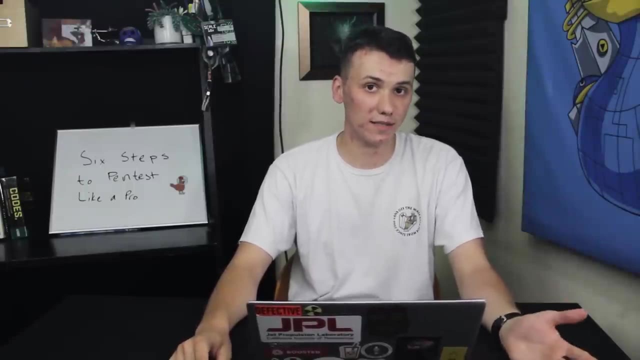 exploitation, but today we're going to be showing command injection. Stage five- post-exploitation, is only possible after a successful exploitation is completed. This is where we use our newfound access to the device in order to raise our privileges or gain permanent access to that. 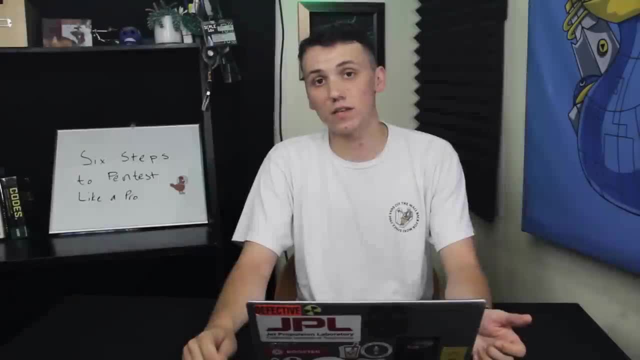 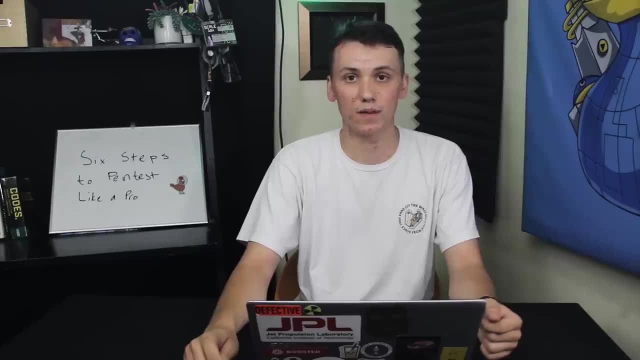 device. The final stage of a penetration test is reporting. This is where we gather all the knowledge that we gained throughout the penetration test, organize it and publish it so other people can be aware of this vulnerability. On this episode of Cyber Weapons Lab, we're going to be targeting 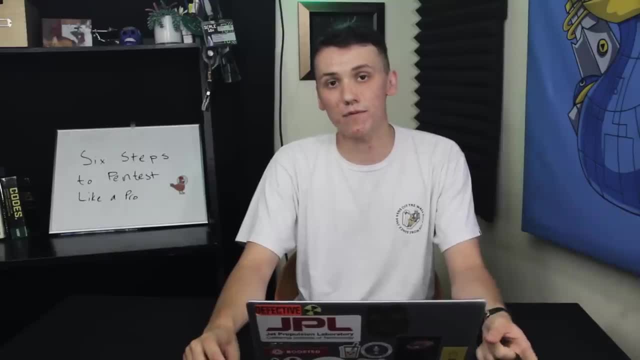 a web server on our local network. We're going to be using NMAP for reconnaissance, we're going to be using Nessus for vulnerability assessment, we're going to be using command injection in order to exploit the device and we're going to be using Postenum in order to elevate our privileges on. 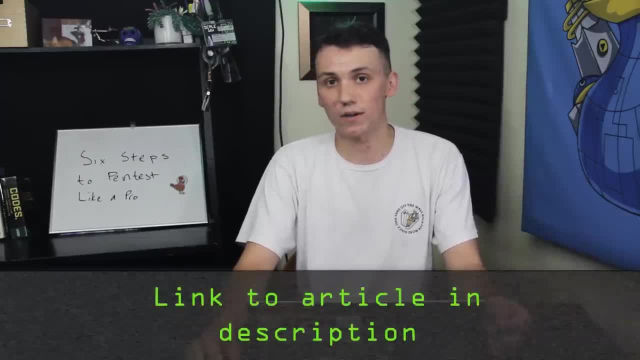 that device. If you have any problems with your device, please contact us. If you have any problems with this tutorial, check out the article linked in the description. All you need to follow this tutorial is a computer to work with. Let's get started. 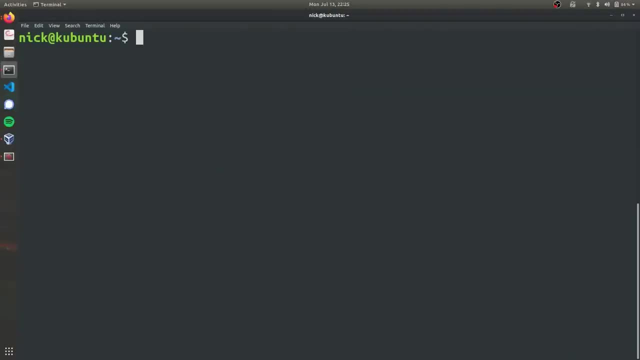 So for the reconnaissance stage we're just going to use a simple NMAP scan And we've covered NMAP before on WonderHowTo and you can check out our tutorials on wonderhowtonobotcom. but I'm just going to show you a real quick one-liner that you can use to 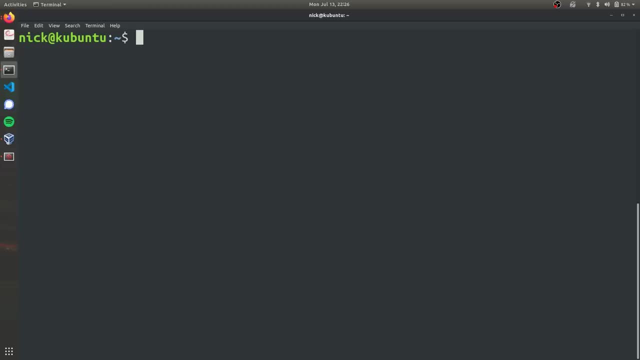 see if there's any open port 80s on your local network. So to do that you just have to type in NMAP and then S capital V for service scan and then you're just going to select the range of IPs that you want to scan. So I'm going to do 192.168.1.1, and we're going to 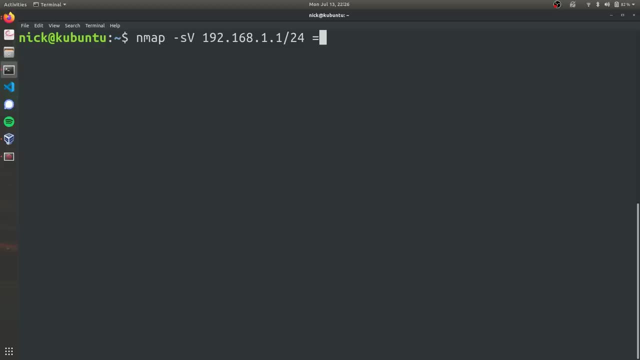 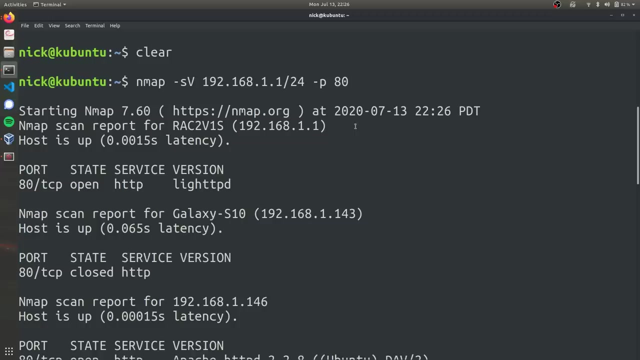 specify our subnet mask with slash 24.. Then I'm going to specify port 80, and I'm going to go ahead and let that run. It's going to take a couple seconds because it's not a huge scan, And after a couple seconds we can see all the devices which are attached to our local network. 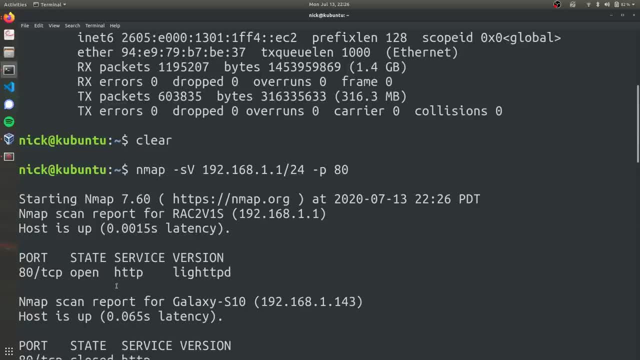 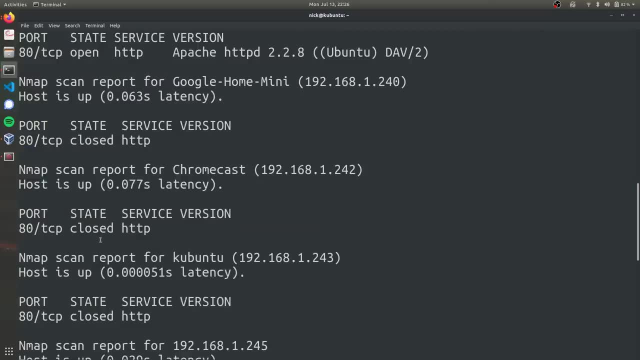 and whether it's open, closed or filtered. So if it's open, that means that port 80 is open to use. If it's closed, that means obviously we can't use port 80. And then filtered means it may or may not be open, but we can't connect to it. 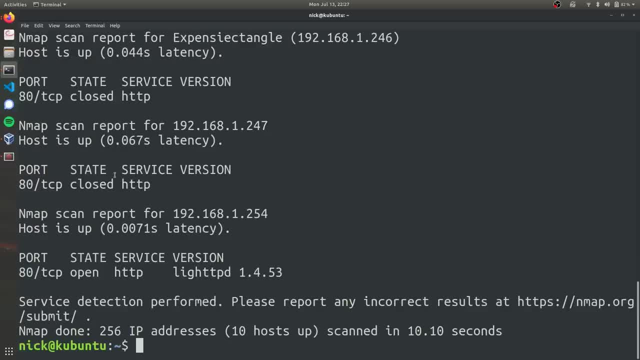 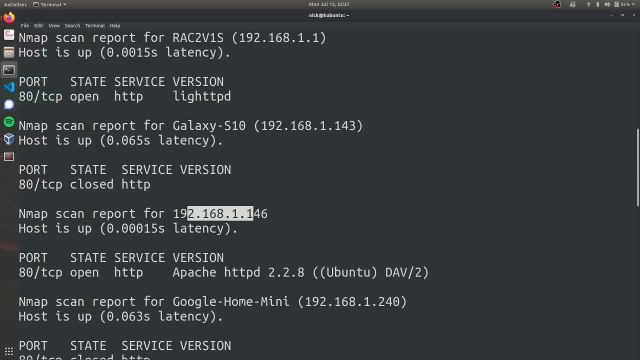 Usually port 80s aren't filtered. That's usually something with SSH or other PCP ports, But today we're going to be interested in 192.168.1.146, and we can see that it's port 80 is open Now. 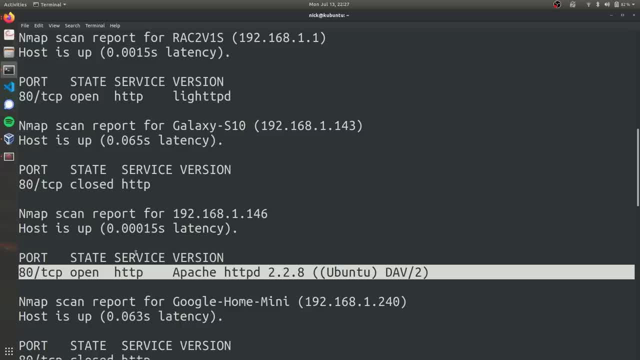 this is a case where I actually have identified that my target is this exact device here, but it's not open. So I'm going to type in 192.168.1.146, and we can see that it's open. But you can use this reconnaissance stage to find any other port 80 device which. 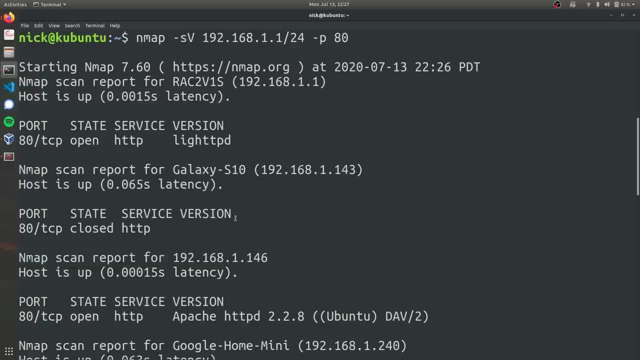 has an open port 80 on your local network. So now that we've used some network reconnaissance to identify our target, we're going to go to the next stage, which is vulnerability assessment. So to do that, we're going to use a tool called Nessos, which has been covered on. 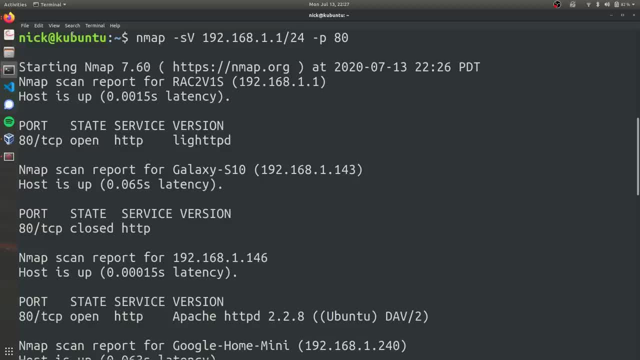 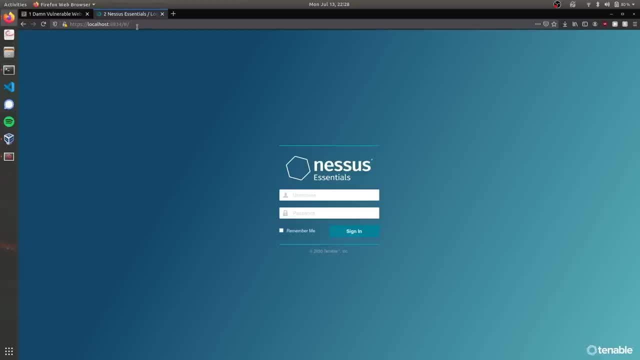 Nullbyte before and that article will be linked in the description as well. So this is going to be assuming that you have Nessos already up and running on your computer, So to navigate to Nessos you just have to open a web browser. I'm using Firefox. 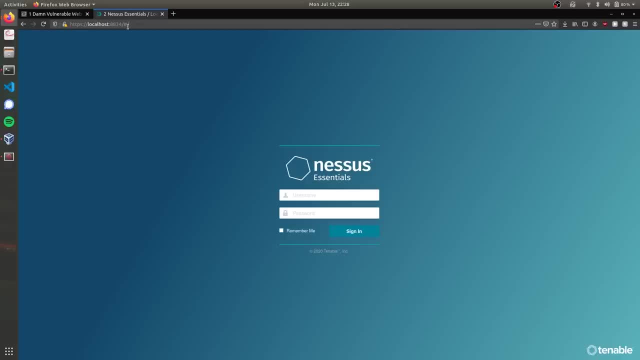 I'm going to type in HTTPS colon- forward slash, forward slash- local host, And then you're going to specify port 8834.. Your web browser might notify you that it could be a security risk to navigate to that address, but you're just going to let it know. it's okay. And once you're here, 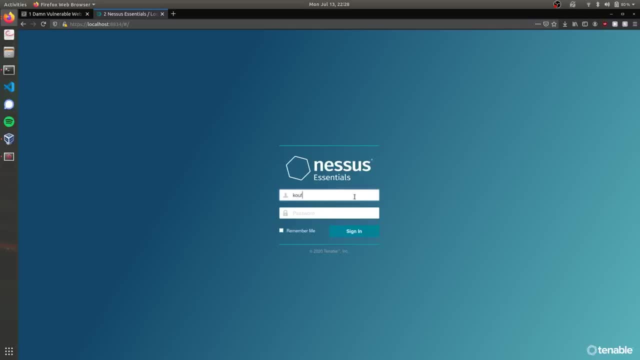 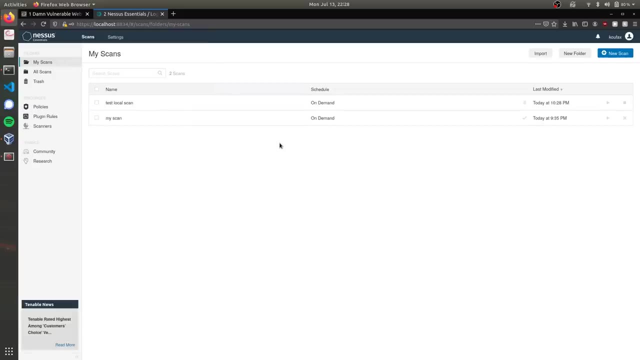 the first time you use Nessos, you're going to have to set up an account. I already have, So I'm going to log in under Kofax And then, once you open the Nessos, the main screen is all the different scans that you've saved or have used previously on Nessos. I've already 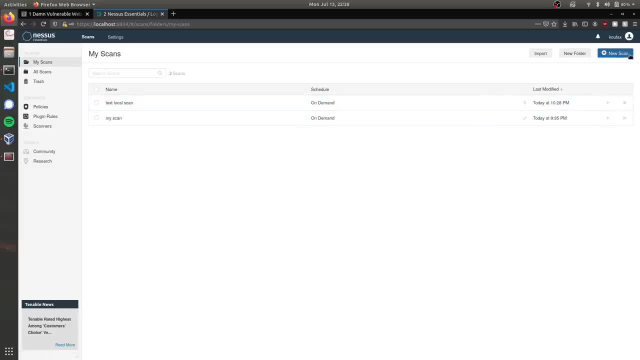 done the scan because it can take a while. but I'll just show you exactly how it works, Exactly how I set it up. So you just press this new scan button and then we're going to do a basic local network scan. We're going to call it null byte test. This is for the video tutorial. 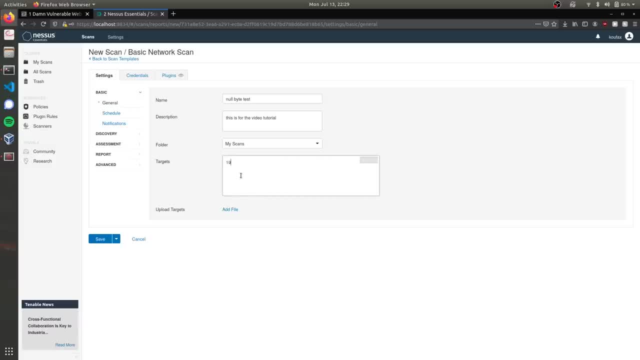 and we're just going to save it in the default folder And you could specify the target that we identified, which is 1.146.. Or you can also do it like we did an Nmap: just leave it at one and then specify the subnet mask 24.. And this will basically leave these first three alone. 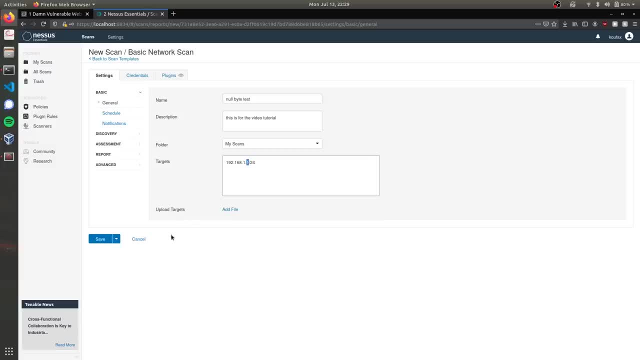 And then just cycle through that last number on our IP. So we're just going to leave it like that, You're going to save it, And then you'll see this null byte test and we can run it, because it's never been run before. So you can launch it And because this is a pretty big scan, it will take a. 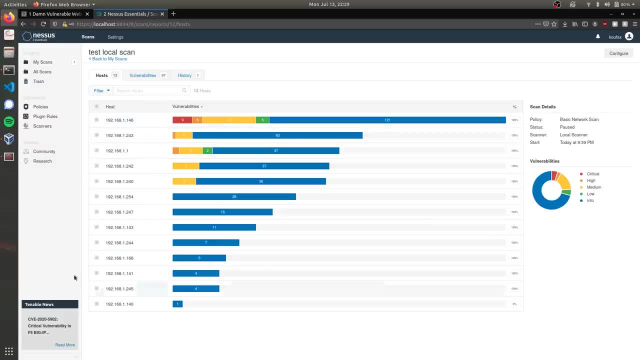 while. So, before I started recording, I ran the scan earlier And, as you can see, my Metasploitable virtual machine has taken up a lot of vulnerabilities, And there's some other devices on my network which might be susceptible to some vulnerabilities as well. So I'm going to go ahead. 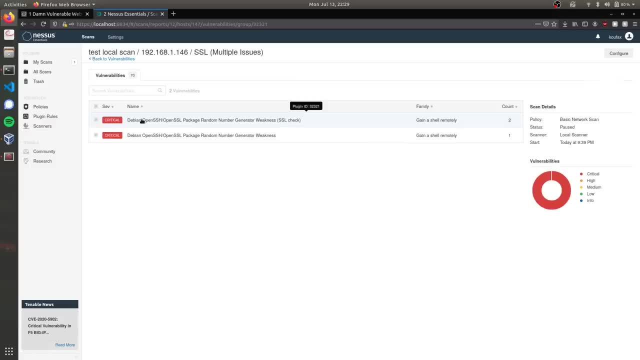 and run it. As you can see, it's using SSL, So there's some issues with SSL, which is usually associated with port 80. And so we know that if we navigate to the web app, then it's probably going to be a vulnerability there. Command injection might be possible. So once you've identified that, 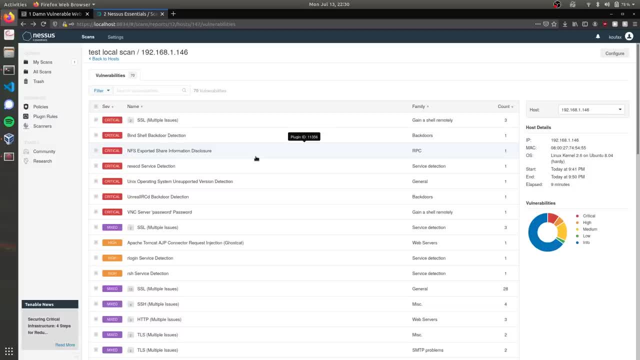 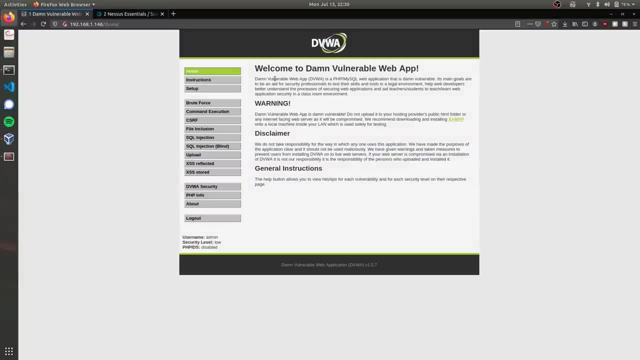 yes, this target that I'm interested in is very vulnerable. you can carry on to the fourth step of the penetration test, which is the actual exploit, the exciting part. So my demonstration for a exploit is just going to be a simple command injection, And so this is a part of Metasploitable 2's. 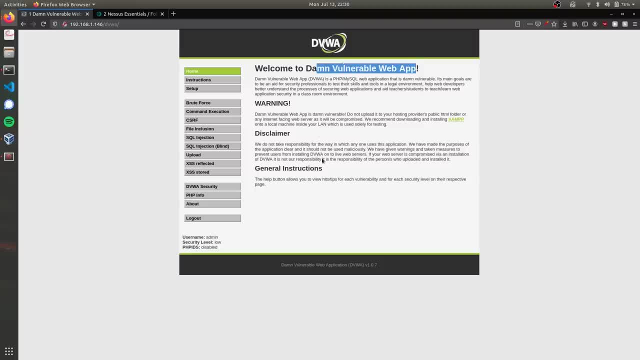 framework, which is the damn vulnerable web app. But this could be a substitute for any web app, It's just. this is just for demonstration purposes. So if, for some reason, a web app allows you to ping IP addresses, then you can take advantage of that and use the computer that you're using to ping. 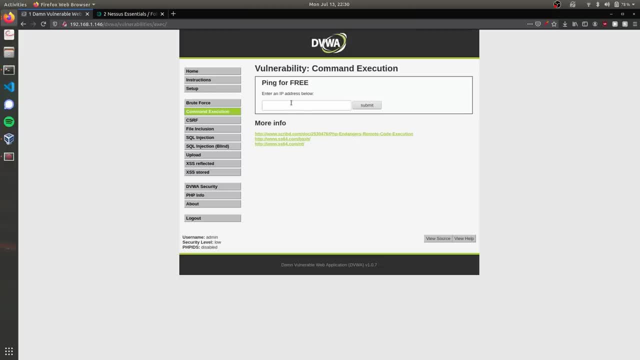 and use it for whatever you want to do. In this case I'm going to create a reverse shell So I can just do a simple scan of the local host which is 127.0.0.1.. And if I submit that, it'll give me. 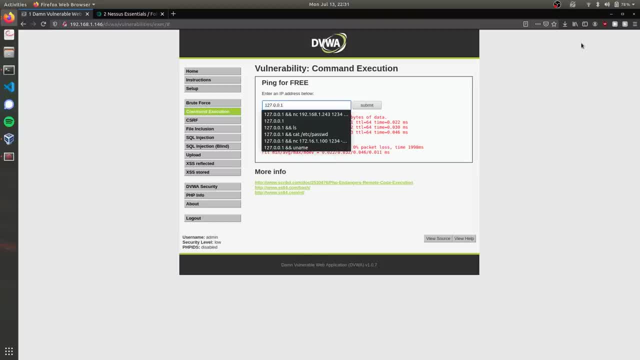 some information back Now. if I specify this remote host and do an ls command, i'm not actually on this computer. i haven't logged into this computer at all, but i'm able to actually see the files on this metasploitable computer without having to put a. 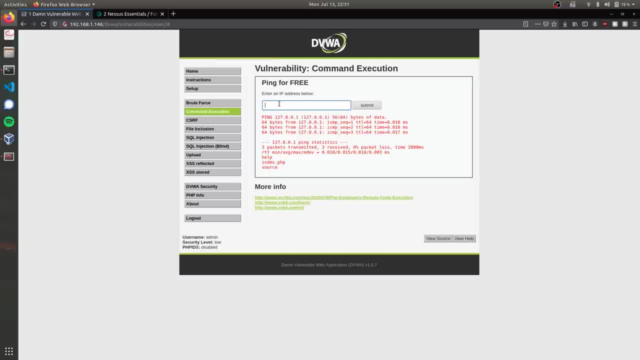 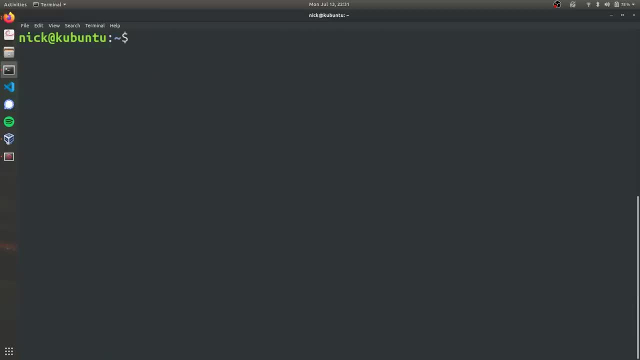 password in or anything. so, because this is not the best way to interact with that computer, let's go ahead and create a netcat reverse shell now. to do that, you're going to have to open up your terminal again, and we're going to create a listening shell on our local computer. so to do that, you just type. 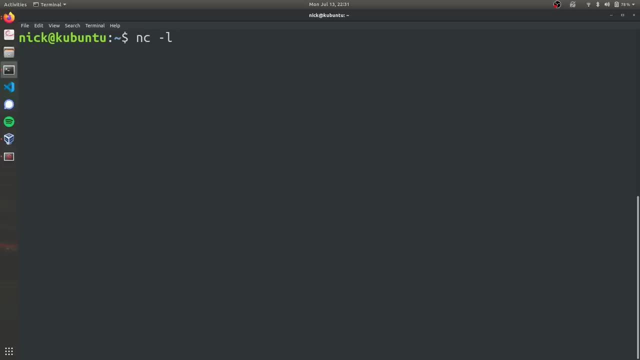 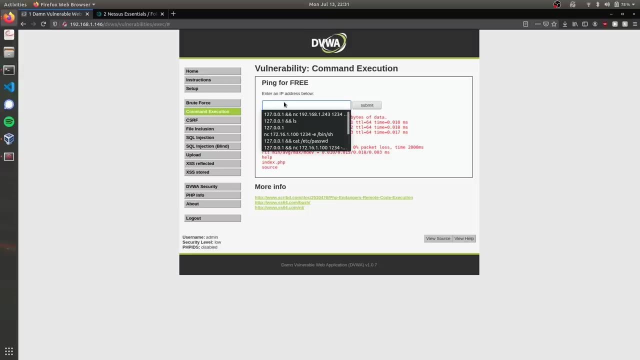 in nc for netcat, tack l for listening and the port you want to listen on. so i'm going to do one, two, three, four. so now it's not going to give you any feedback, it's just already running the second. you do that. so now we're going to specify a local host and then we're going to do: um, i typed in the 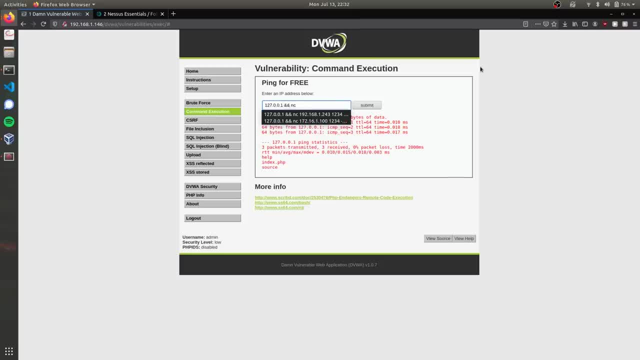 command earlier, as you can see, to test. but you're going to type in ncat and then you're going to specify the ip address of your local computer where you're sending this to. so i already know that ip is 192.168.1.243. 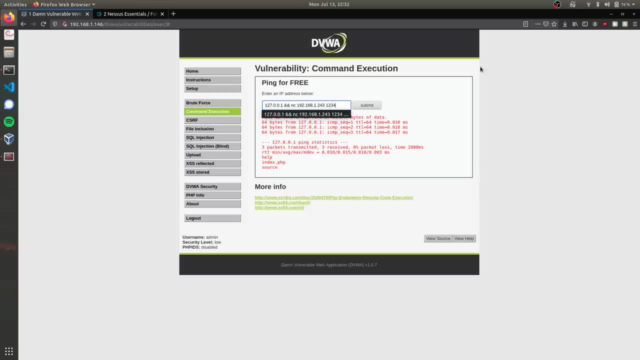 and then you're going to specify the port, which is one, two, three, four, and then we're going to specify tack e for execute and we're going to create a terminal in the netcat shell so you can go ahead and submit that it might take a second or two. and then now, if we go back to our terminal, 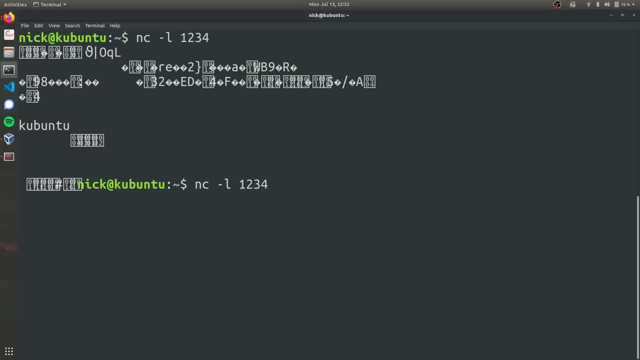 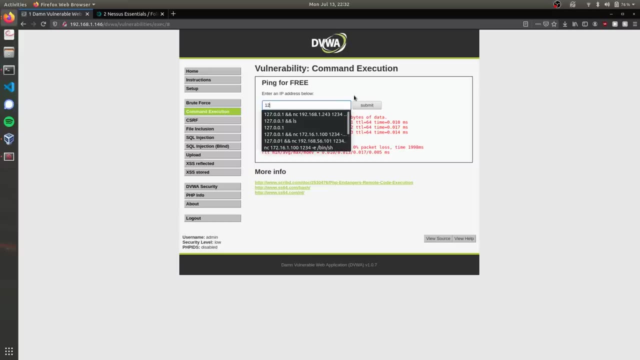 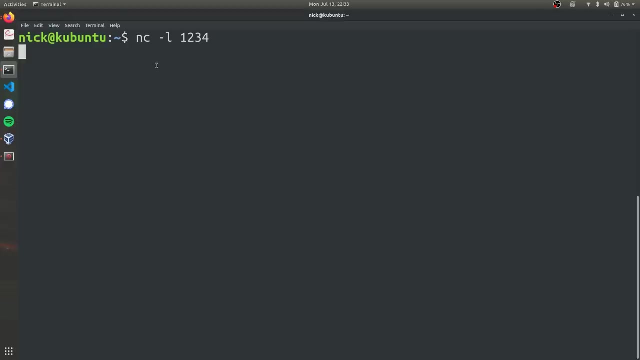 you can see, some funky stuff happened. it actually closed, so let's actually try that again. oops, not clear. we're going to try listening again and then we're going to do one, two, seven, one, six, eight, two, four, three. yeah, that all looks right and if you type in, it's still loading. so now, if you do, who am i? you get this www attack data. 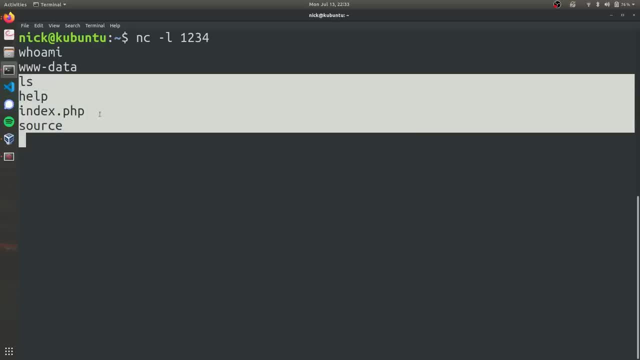 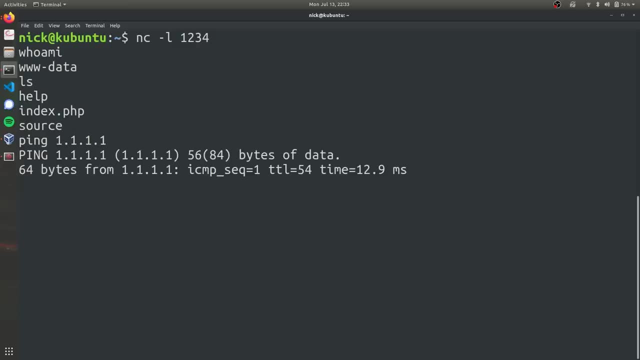 and if we do ls here, we can see that these are the files actually on the metasploitable computer and now we basically have a complete shell. so we can ping from here now and you can see it's getting this data, and then i actually enclosed it. but from here you can move on to the post. 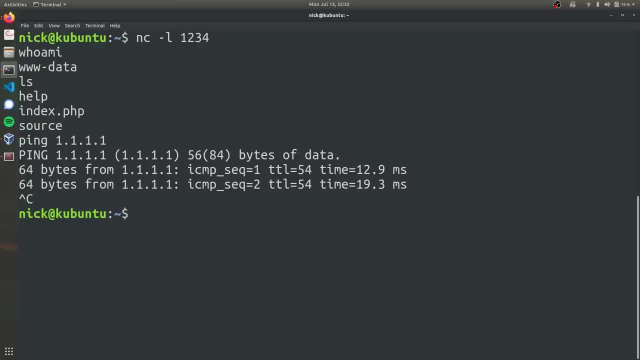 exploitation phase of the attack. i'm going to be using a previous video we did on a tool called postenum, which you can see is going to be a little bit more complicated, but i'm going to be using a local device and i'm going to use it to scan a local device and find any vulnerabilities that 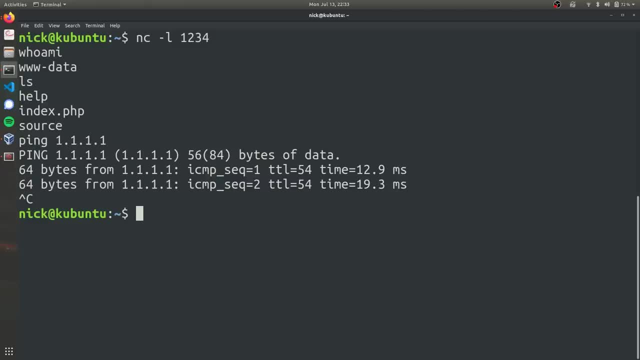 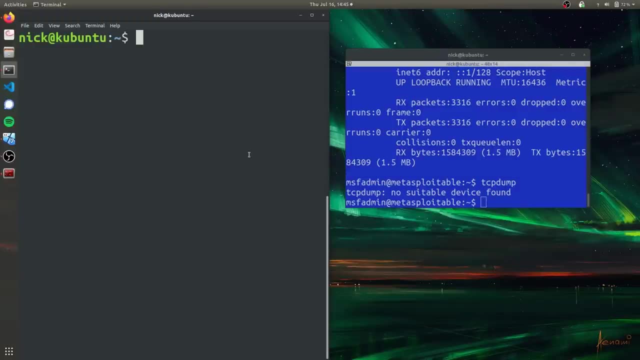 that device is susceptible to, so you can either raise your privileges or create a permanent back door into that computer. so, assuming that you've been able to access a the target computer, either by creating a reverse shell with command injection or whatsoever, we can go ahead and install. 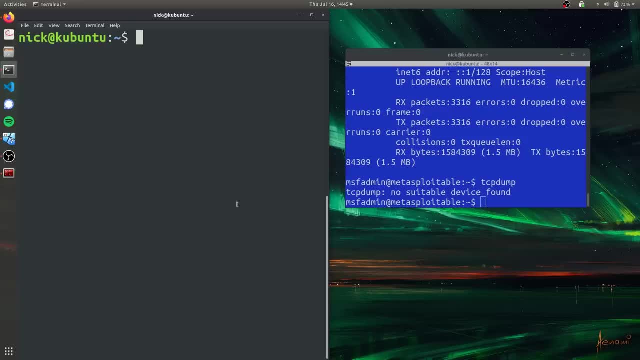 posting them onto the target computer. but first let's download it onto our computer. first, and just for reference. this left black and green terminal is going to be representing my local computer and this blue and white terminal on the right hand side going to be representing the targets computer. this is my reverse shell into: 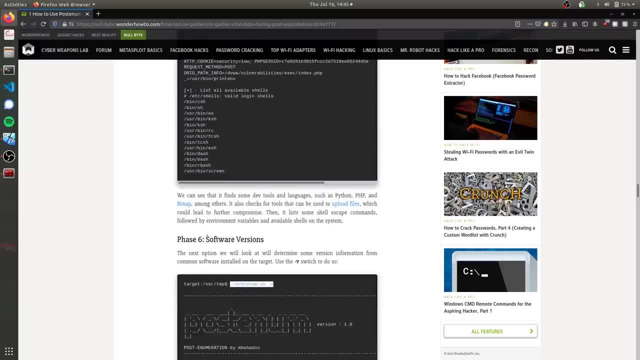 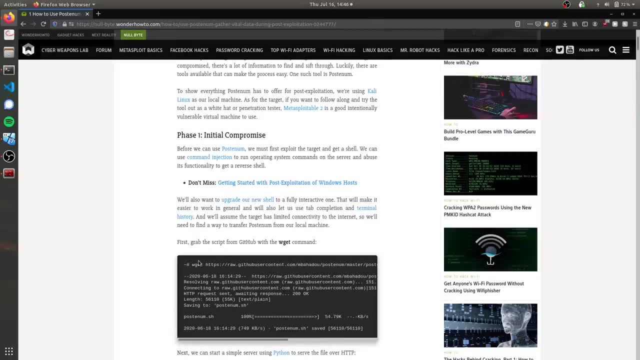 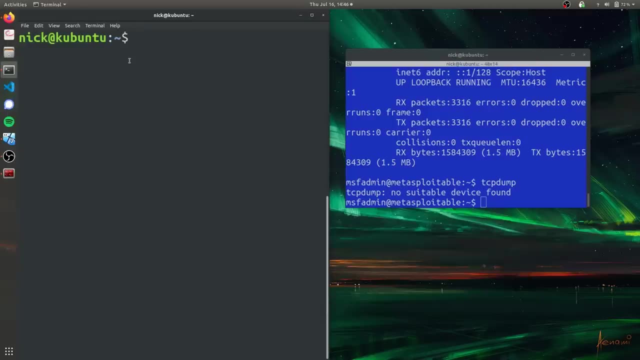 that computer. so if you go ahead and navigate to the nullby article for postenum- and you can, if you scroll up to one of the first steps, actually we can download postenum by using this wget command, just downloading the script directly, and we're gonna go ahead and install it onto our local machine. okay, 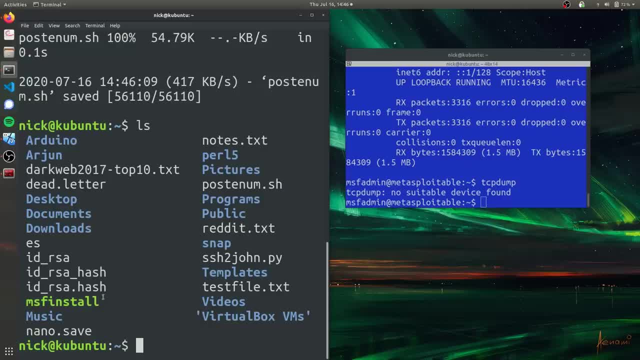 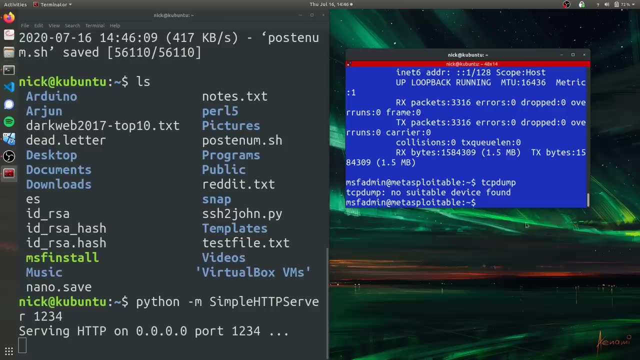 and then now we can see that we have postenum somewhere. there it is postenumsh, and let's go ahead and set up a simple HTTP server on port one, two, three, four, okay. and then now, if we go to our target computer and now we can grab the postenumsh from our local machine- oops, and you got to. 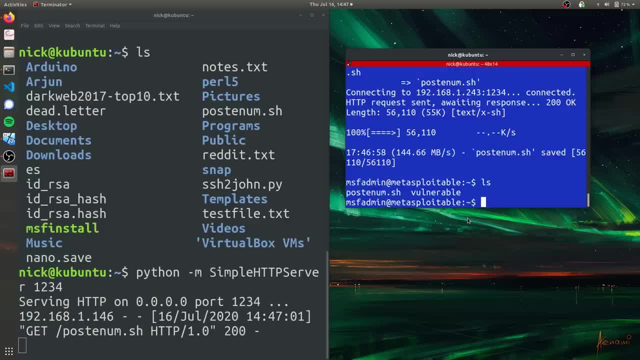 specify the port. of course, there we go. now, if we look on this local machine, we have postenum. so we can go ahead and try to run postenum like we would on our local machine. so we can go ahead and try to run postenum like we. 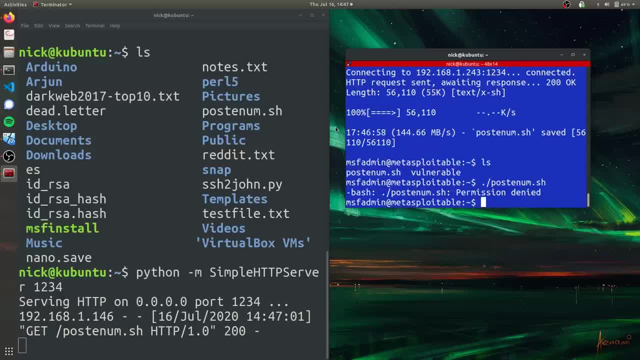 would on our local machine so we can go ahead and try to run postenum like we. would a normal bash script, but more often than that it's not gonna work- would a normal bash script, but more often than that it's not gonna work because it doesn't have execute privileges. so to do that you just have. 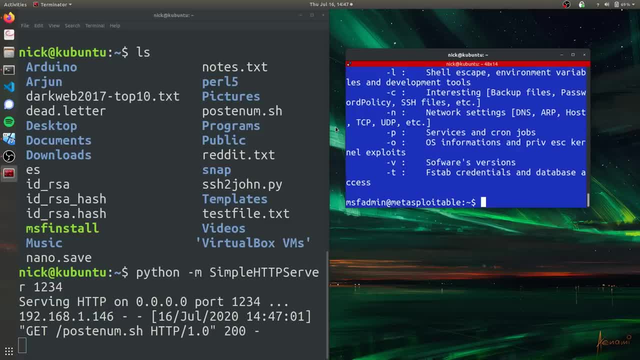 because it doesn't have execute privileges. so to do that you just have to use chmod, okay, and then now we can go ahead and try and run it like we did. to use chmod okay, and then now we can go ahead and try and run it like we did. 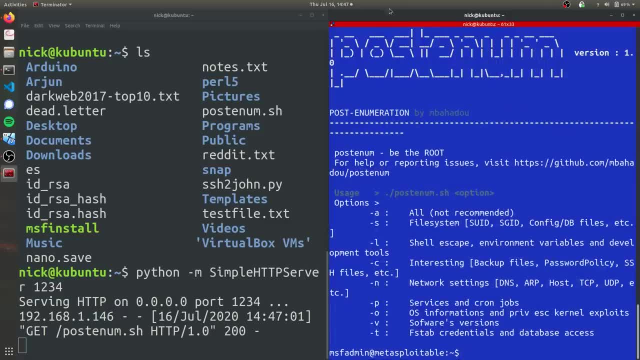 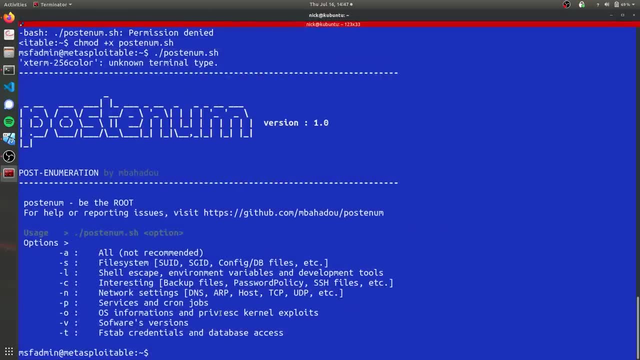 earlier. I'm gonna go ahead and make this bigger and, as we can see, postenum is earlier. I'm gonna go ahead and make this bigger and, as we can see, postenum is working now. so let's go ahead and I'll show off a couple features. so first we 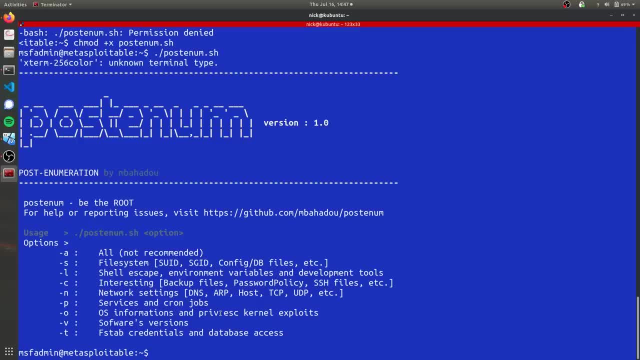 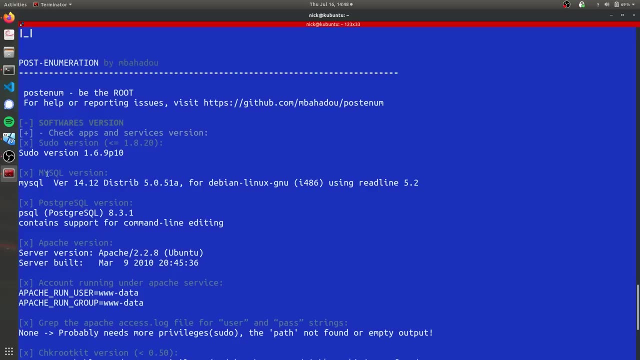 working now. so let's go ahead and I'll show off a couple features. so first we can see what versions of software are actually installed on this computer. so can see what versions of software are actually installed on this computer. so is run posting them: tech V, oops, dot sh. and we can see versions for mysql Apache. is run, posting them: tech V- oops dot sh. and we can see versions for mysql Apache is run, posting them: tech V- oops dot sh. and we can see versions for mysql Apache Java and we can see if any of these are Java. and we can see if any of these are. 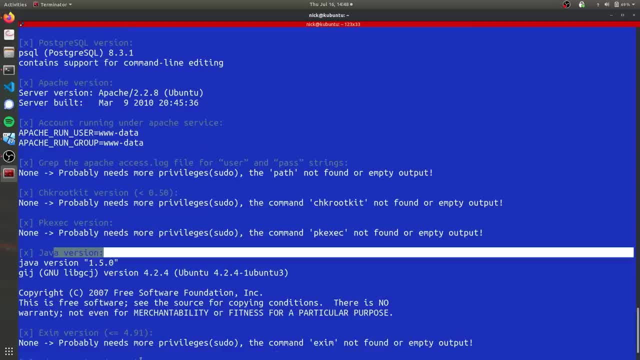 Java and we can see if any of these are old, outdated and vulnerable for old, outdated and vulnerable for old, outdated and vulnerable for exploitation in 2020 or whatever year exploitation in 2020 or whatever year exploitation in 2020 or whatever year you're doing this in. and then one more: you're doing this in, and then one more, you're doing this in, and then one more thing we can do is we can see what thing we can do is we can see what thing we can do is we can see what development tools are available to us. on. 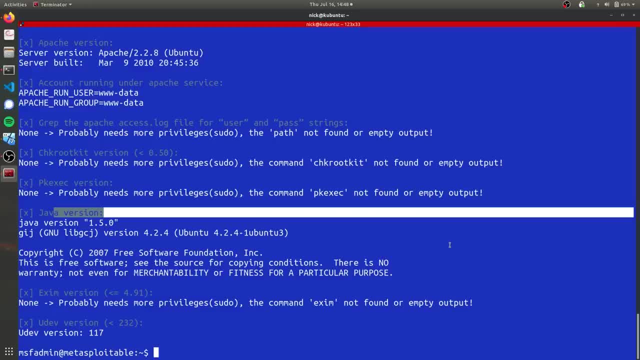 development tools are available to us on. development tools are available to us on this computer, whether PHP is installed this computer, whether PHP is installed this computer, whether PHP is installed on this with a pearl or Python, so we can on this with a pearl or Python, so we can. 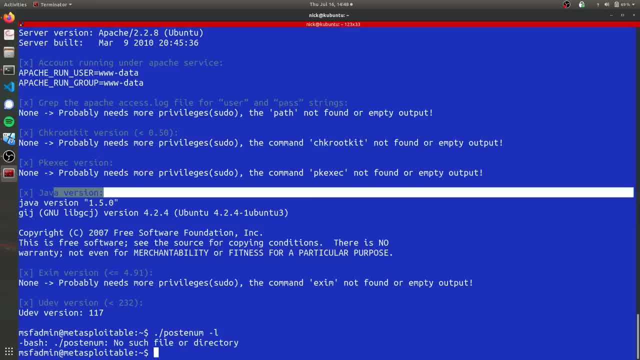 on this with a pearl or Python, so we can know what kind of scripts can actually know, what kind of scripts can actually know, what kind of scripts can actually be applied to this computer. oh, and you be applied to this computer. oh, and you be applied to this computer. oh, and you gotta specify that it's a ship flash. 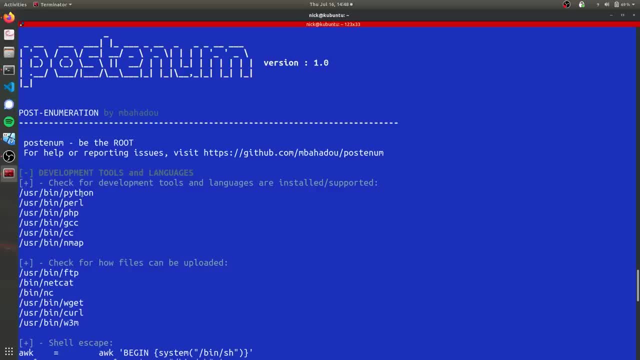 gotta specify that it's a ship flash, gotta specify that it's a ship flash file. and so we got some interesting file. and so we got some interesting file and so we got some interesting information. we can see that Python pearl information. we can see that Python pearl. 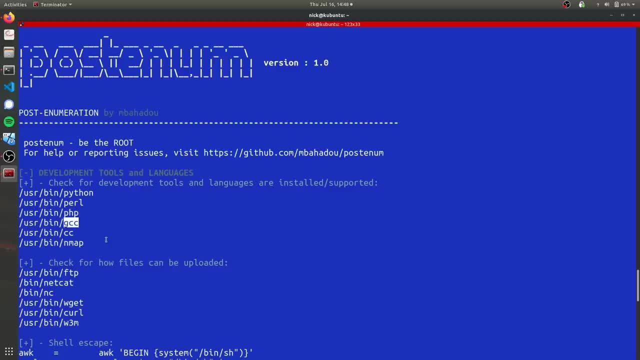 information. we can see that Python, pearl, PHP GCC, which is a C++ compiler, CC, PHP GCC, which is a C++ compiler, CC, PHP GCC, which is a C++ compiler, CC, which is a C compiler, and nmap are all which is a C compiler and nmap are all. 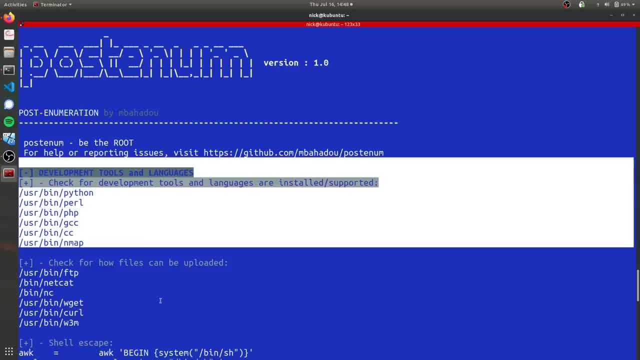 which is a C compiler, and nmap are all installed on this computer. so if we have installed on this computer, so if we have installed on this computer, so if we have a Python script, that we are ready to a Python script, that we are ready to a Python script that we are ready to deploy, that we, you know, is pretty- 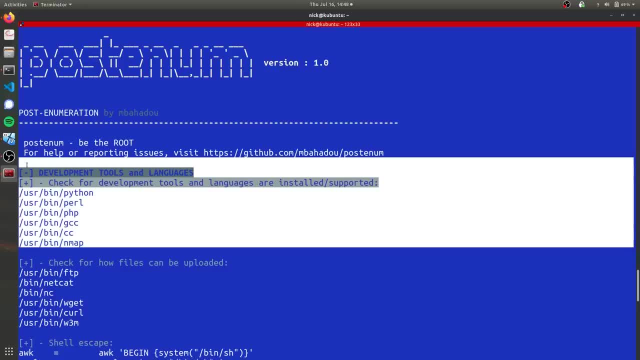 deploy that we, you know is pretty, deploy that we, you know, is pretty effective at escalating user privileges. effective at escalating user privileges, effective at escalating user privileges, then we know that we will be able to. then we know that we will be able to, then we know that we will be able to deploy onto this computer- see how files. 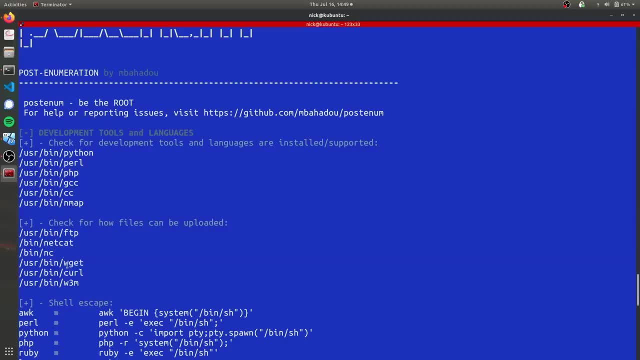 deploy onto this computer. see how files deploy onto this computer. see how files can be uploaded. we can use FTP. netcat can be uploaded. we can use FTP. netcat can be uploaded. we can use FTP netcat, wget, which is what we use to actually get wget, which is what we use to actually get. 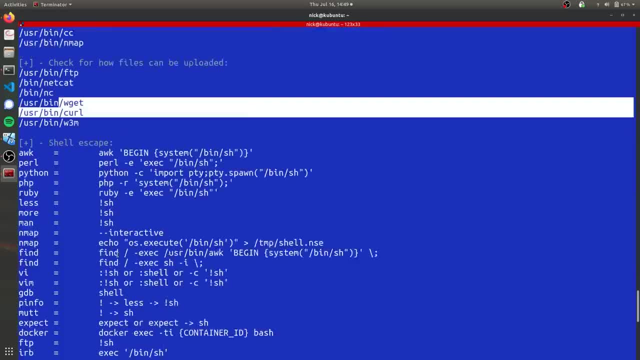 wget, which is what we use, to actually get posted them onto this computer curl. posted them onto this computer curl, posted them onto this computer curl. it's all that is available to us and we. it's all that is available to us and we. it's all that is available to us. and we can see what type of shell terminal. 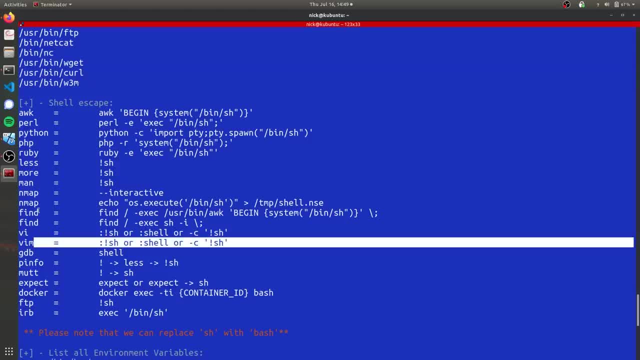 can see what type of shell terminal can see what type of shell terminal tools are available to us. so VI and vim tools are available to us. so VI and vim tools are available to us. so VI and vim are installed and map is installed. Ruby are installed and map is installed- Ruby. 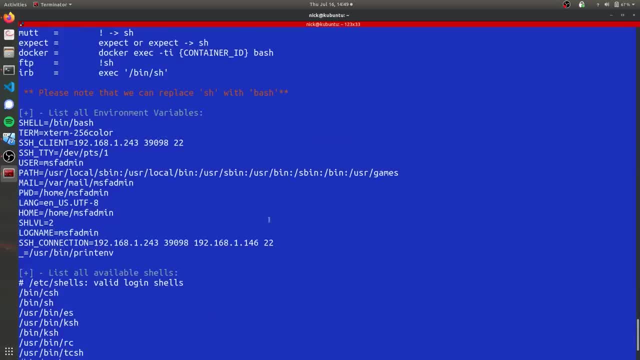 are installed and map is installed, Ruby, which wasn't specified earlier, and we, which wasn't specified earlier, and we, which wasn't specified earlier, and we can see where all of these environment can see, where all of these environment can see where all of these environment variables are actually installed in. 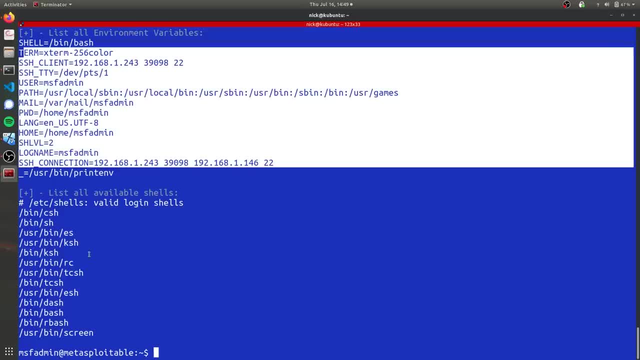 variables are actually installed in. variables are actually installed in case we mess with that and yeah, so case we mess with that and yeah, so case we mess with that, and yeah. so that's just the basics of things you can. that's just the basics of things you can. 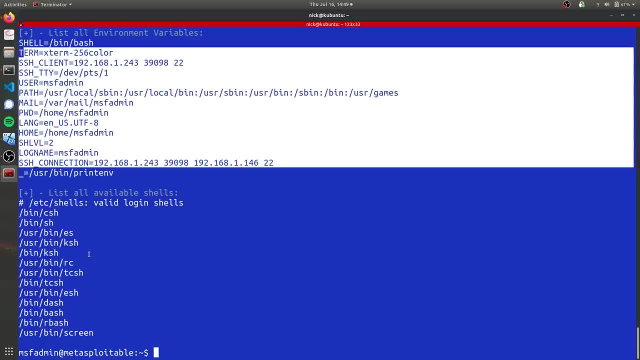 that's just the basics of things you can do with posting them to escalate your do with posting them. to escalate your do with posting them to escalate your privileges in the post exploitation privileges in the post exploitation privileges in the post exploitation stage of a penetration test, if you like. 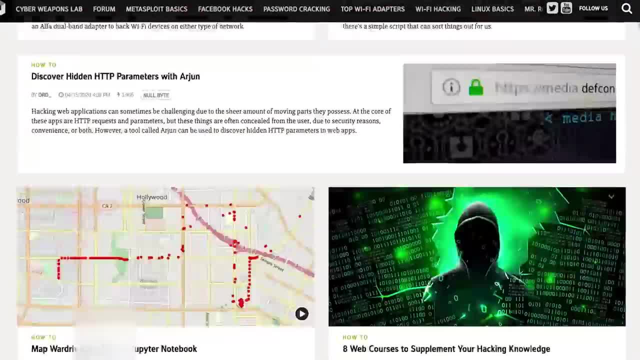 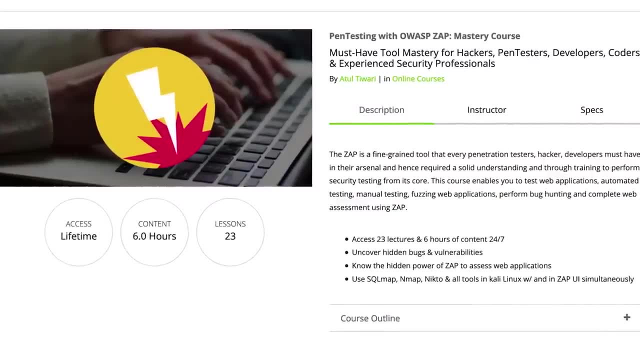 stage of a penetration test. if you like stage of a penetration test, if you like this tutorial, be sure to check out our this tutorial. be sure to check out our this tutorial. be sure to check out our website, where we have hundreds of free website, where we have hundreds of free.